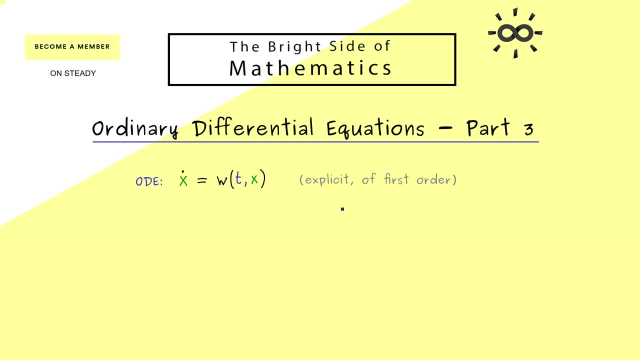 of this form is called explicit and of first order. This means that we only have the first derivative in the whole equation and we only have the first derivative in the whole equation, And the first derivative is also alone on the left hand side. However, i can already tell you. 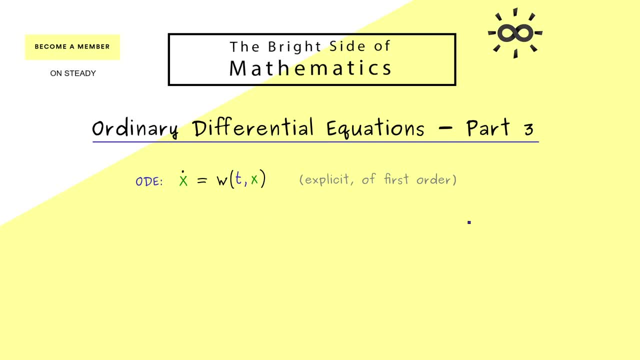 that in the next video we will show that this is not really a restriction. Indeed, we will see we can simplify that even more without losing generality. And in order to see that, let's first look at some examples here, And the first one here should be the ode x. dot is equal to lambda x. 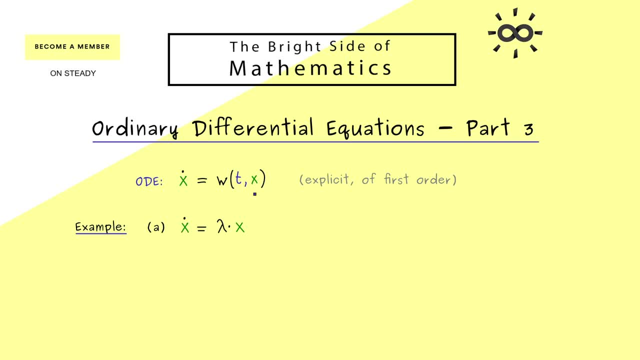 So a very common example. What we should see here is that the function w does not depend on t, Hence the independent variable, the time variable, does not occur in the equation. Therefore we introduce a new name for such odes: They are called autonomous. On the contrary, we can immediately think of an example. 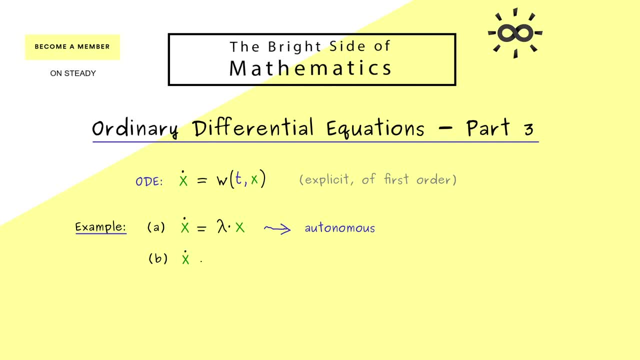 which is not autonomous, Namely x dot, is equal to t. There the first variable, t, will change the value of the function w. Hence this one is an ode, but not an autonomous ode. And of course this notion can also be used for a system of odes, For example in two dimensions. So here x dot is equal. 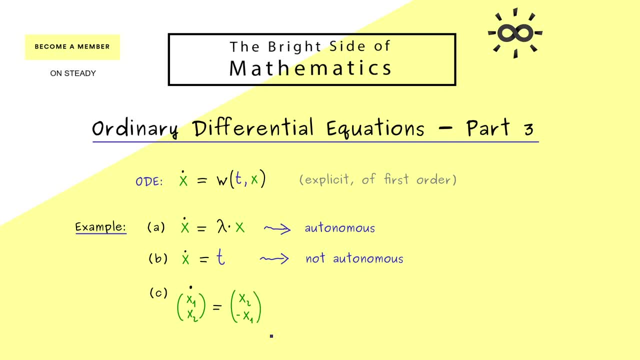 to x2 and minus x1.. So you see, there is no t on the right hand side here. Hence the whole system is also called autonomous. Indeed exactly that These systems will be the interesting ones, so let's consider them for the rest of the 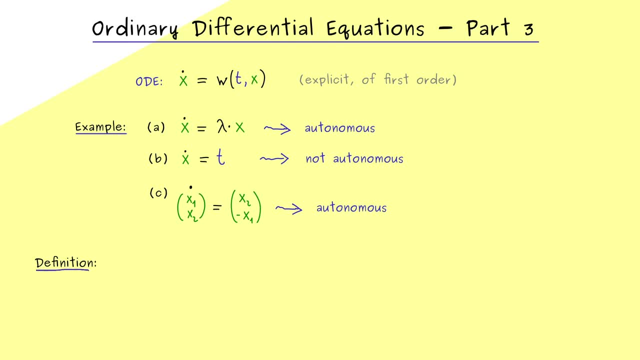 video, And of course we have to put this into a new definition. In fact, we want to keep it short and just call it an autonomous system. So it means we have a system of ODE's, and the function w on the right hand side does. 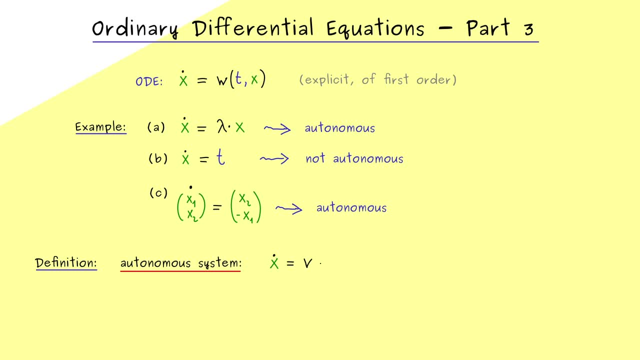 not depend on t. Therefore we can just write it as a function v only depending on x. Moreover, you know we have a whole system, so this can be a vector equation, which means the function v maps Rn to Rn. However, in general you know, v can have a domain, so it maps u into Rn. 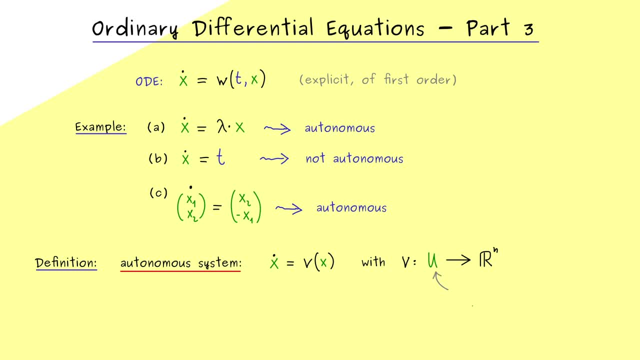 But of course u should then be a subset of Rn as well, And indeed often we will choose u as an open set. Moreover, I would also say that all the times you see that v is at least a constant, So it is a continuous function defined on u. 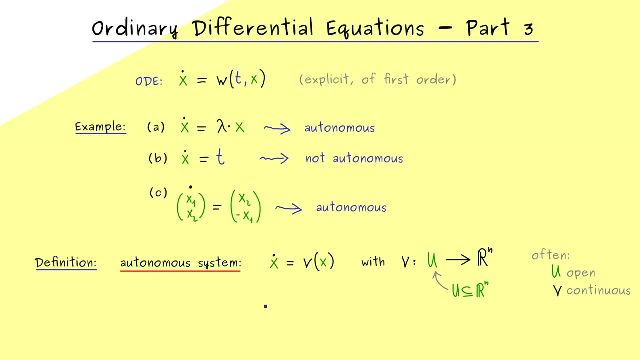 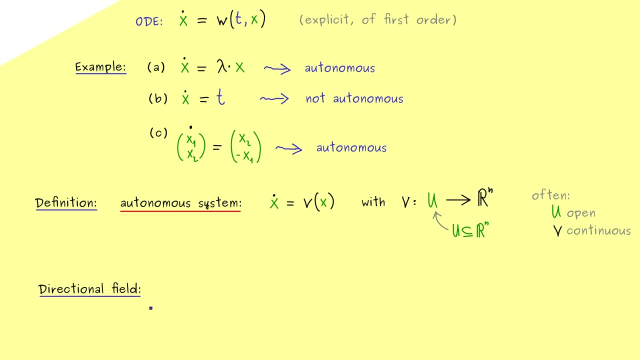 Ok, but now the point is, such an autonomous system can be nicely visualized And this is done by the so called directional field. I would say this is easy to understand because it is simply a plot of our function v. So you could say this is a vector field which visualizes the function v. 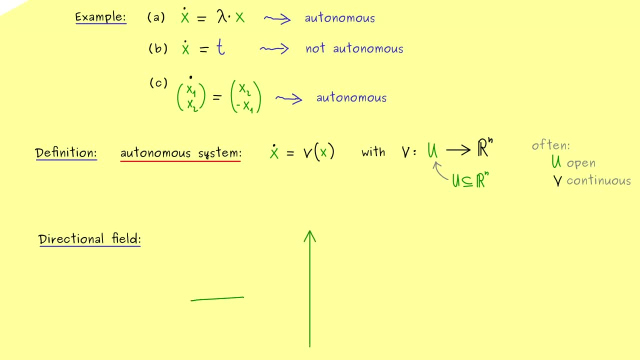 Therefore you would start with the domain u, which is a subset of Rn, So for example, it could be the whole R2.. Hence here lets visualize an example where v maps R2 into R2.. So if you choose any point p in this coordinate system, the resulting value of v will also 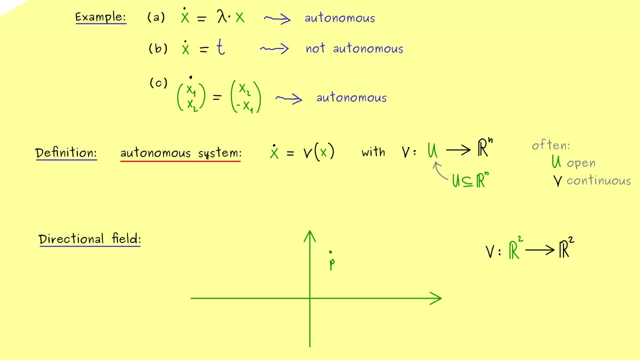 be a vector, And this vector we can simply visualize as an arrow starting at p. Now, this is a common way to explain a vector function like v. And this is the vector function. And now, of course, the important fact here is that you could do it at any other point in this coordinate system. 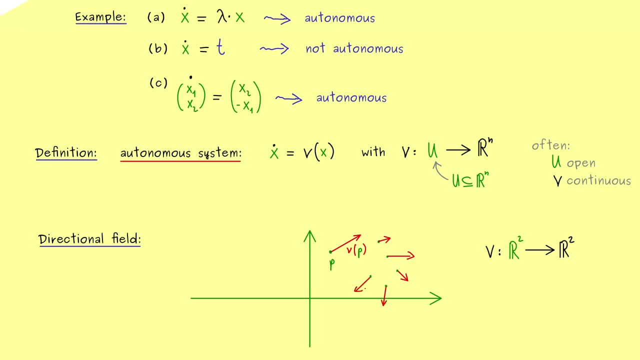 And then you simply have a picture with a lot of arrows. However, we now call it the directional field of the ODE, because it explains what solutions have to do. Namely, the ODE, the whole system of ODEs says that, at a given point, this vector is exactly the derivative of the solution. 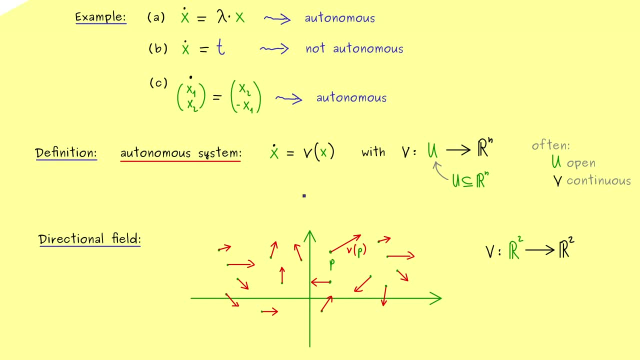 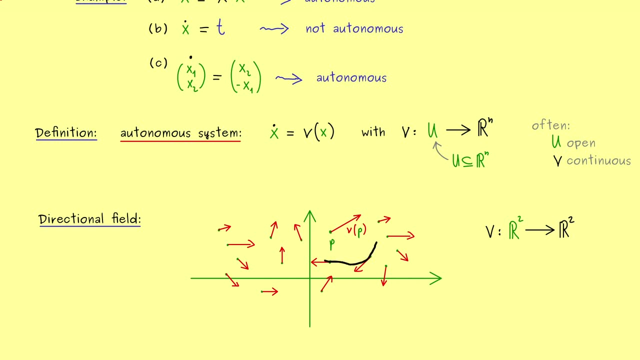 Indeed, this fits nicely in with the pictures of the orbits we had in the last video. Please note: an orbit would be the image of a solution here in our domain. However, now we know this can only be a solution of our system if, at each point, the vector we see is a tangent for this curve. 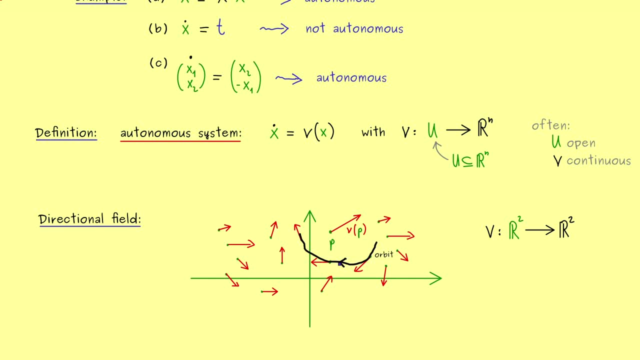 Simply because at each point the vectors here tell us in which direction the solution should flow. In other words, if we plot the directional field of this vector, function v, we can already see what the solutions can do and what they can't do. 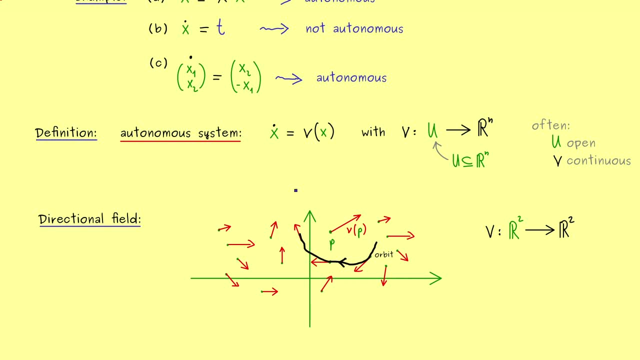 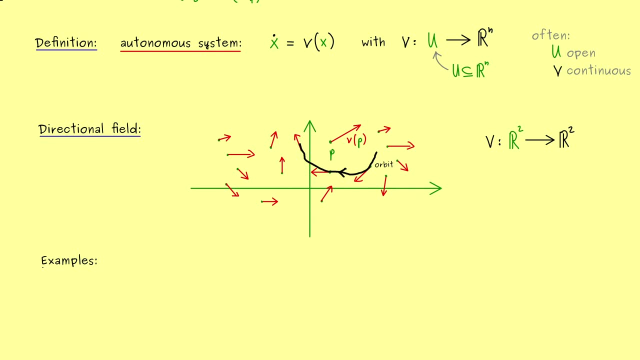 Therefore this whole thing here is already very helpful to see the behavior of possible solutions of the ODE. But of course this whole procedure here we should explain with examples, And first let's start with a one-dimensional example. So x dot should be equal to the sine of x. 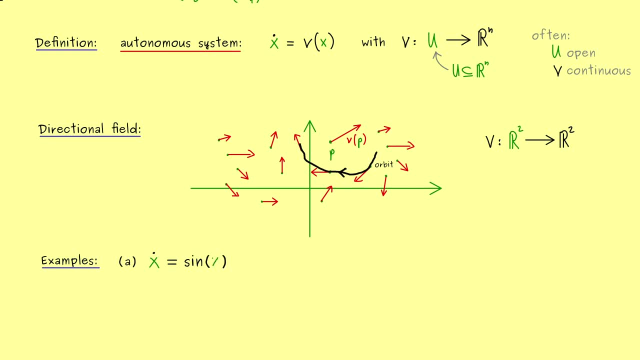 So not too complicated, but we also realize that we don't see all the solutions immediately. However, we can recognize that v is defined on the whole real number line, And this means that our directional field is now just a one-dimensional picture. 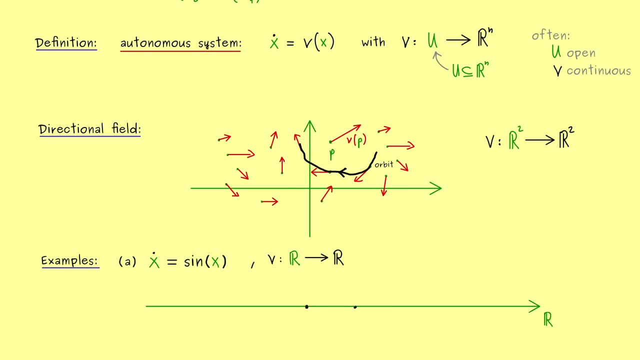 Hence for the arrows we want to draw in. there are only two possible directions To see what happens here. let's look at some important points like 0, pi over 2, pi, and so on. Of course, we choose exactly these numbers because of the sine function. 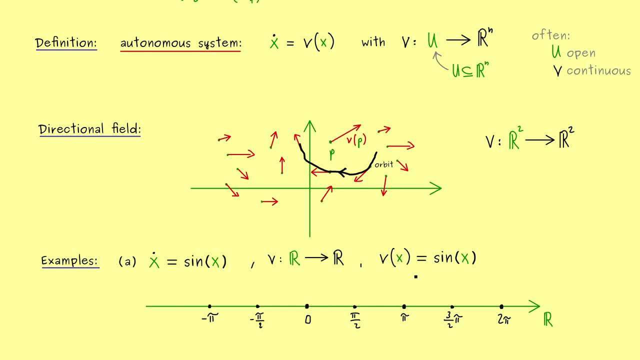 So, for example, if we put pi over 2 into our function v, we get out 1.. In other words, we have an arrow of length 1, that points to the right. On the other hand, if we choose 3 over 2 times pi and put that into our function v, we get out minus 1.. 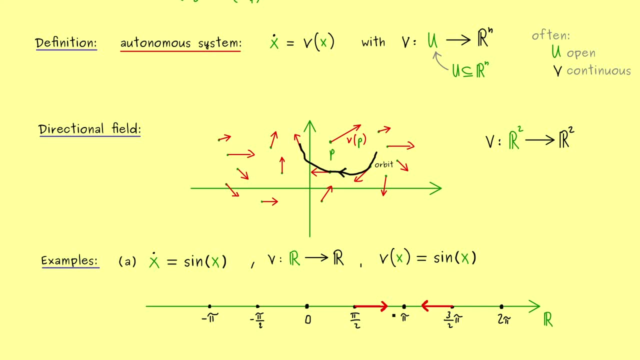 So an arrow that points to the left. So you see, this is what we could do for all points on the real number line, and then we get the whole directional field. So, as another example, if you choose a small number, positive number- here on the right of 0, we also get an arrow that points to the right. 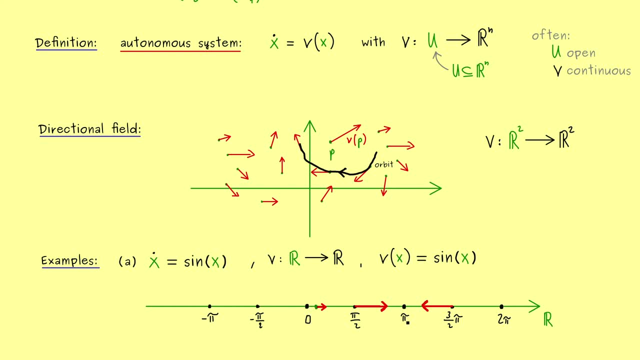 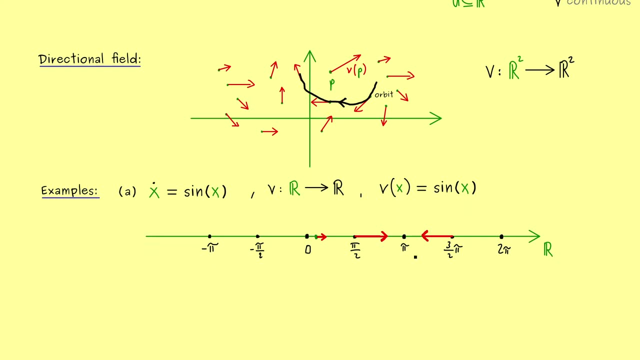 However, please note, at the point 0 and at the point pi we simply get out 0. This means that at these points there is no arrow pointing anywhere, But exactly that is immediately an important information for the solutions. 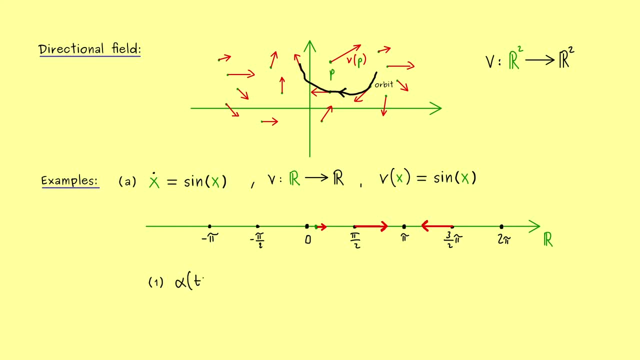 So, for example, you could take a solution: alpha t, that is always 0. So it means alpha t vanishes, no matter which t you put in. And now we can simply check that this is indeed a solution. 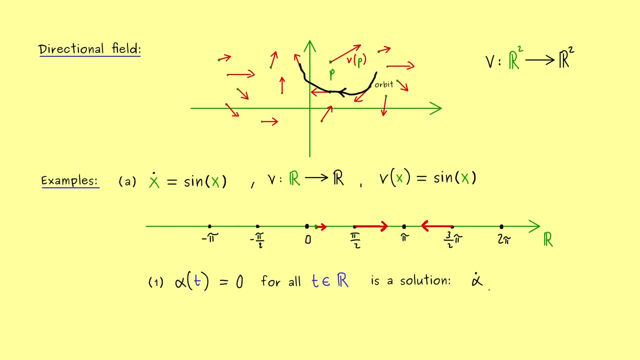 This is not hard to do. you simply put alpha into the ode. So we want that alpha dot of t is equal to 0.. So this is what a solution has to fulfill for all t, And here we don't have a problem because the derivative is 0, and sine of 0 is also 0.. 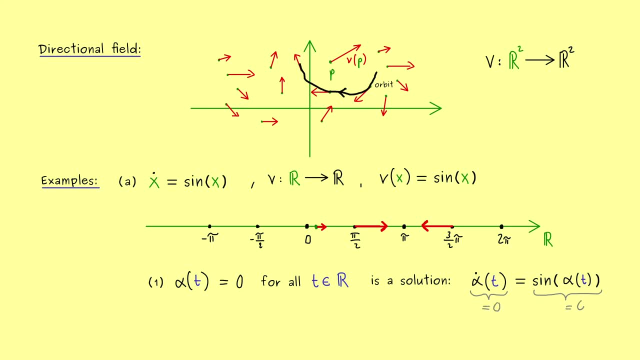 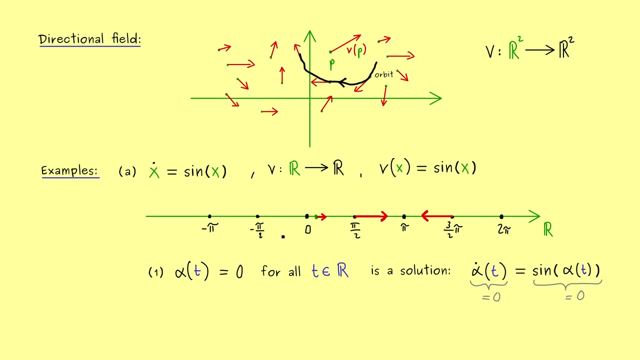 So here we simply have: 0 is equal to 0.. Now, this is important to remember. this always works if you find a point in the directional field that has no arrow at all, And therefore we can immediately give a second solution. alpha. 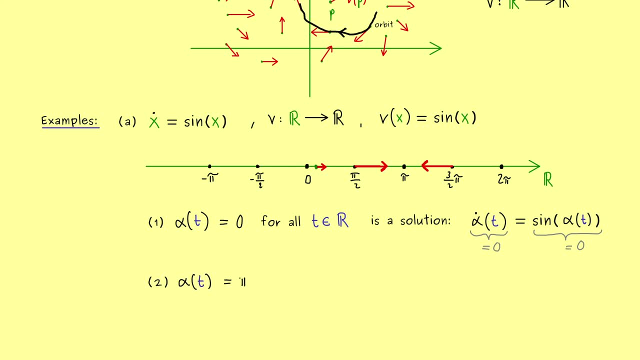 We simply choose it as the constant function with value pi. Indeed, with the same reasoning, this is also a solution, because the derivative is 0, and sine of pi is 0.. And the important fact is, this claim holds for all t in R. 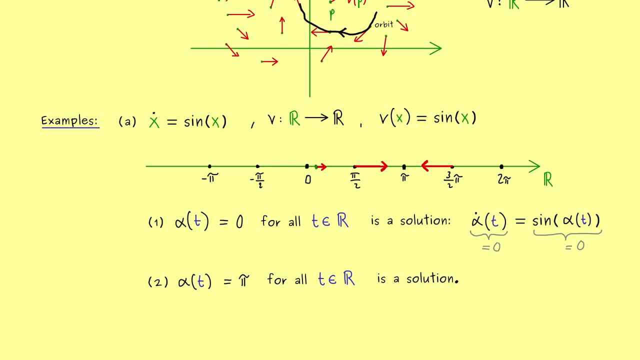 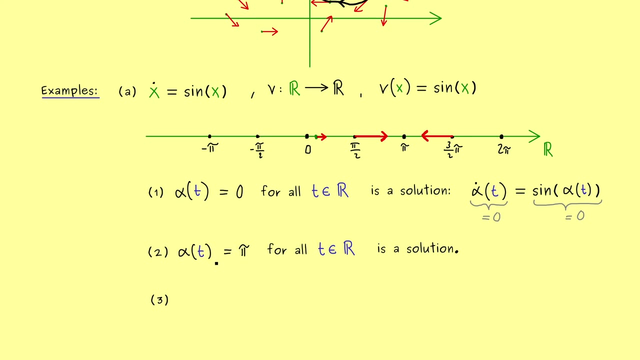 In other words, you see, here we have solutions that stay with their orbit just on one point, And for this reason these points in the picture are called alpha, These points in the picture are called stationary points. However, the directional field does not only tell us about the constant solutions here. 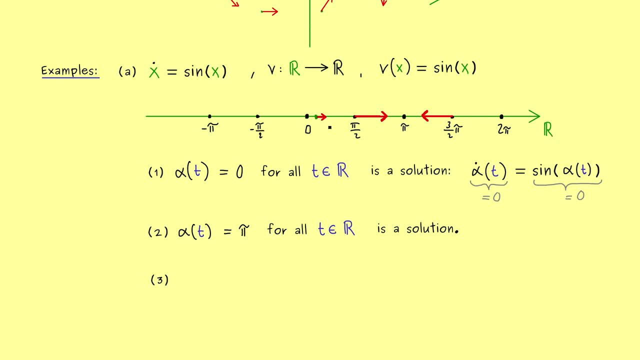 Moreover, you should see, we also get information about the solution that lies in here. In particular, we can look at the solution that hits the value pi over 2.. There we know, if we now increase t, we have to go to the right with the solution. 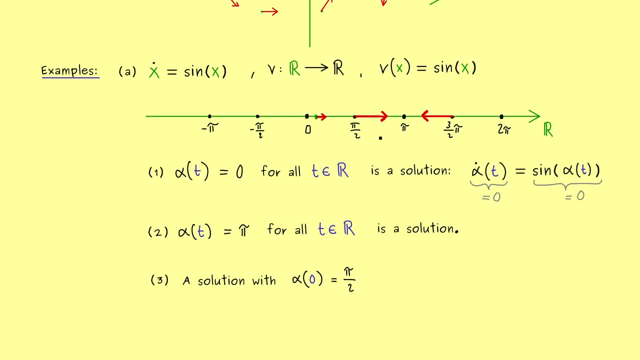 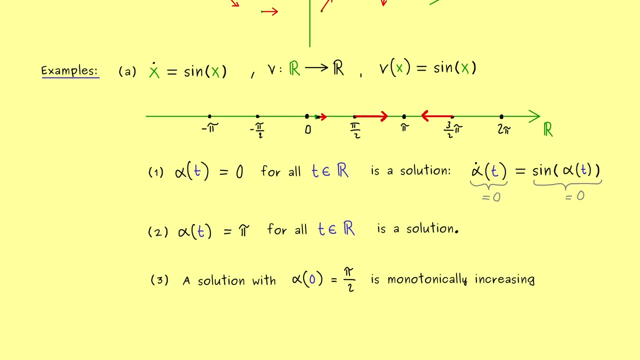 Therefore, we can directly conclude that the solution inside this interval has to be monotonically increasing. Moreover, we also see that we can't exceed the value pi in the end, because pi is a stationary point. This means if we go with t to infinity, we will approach this value pi. 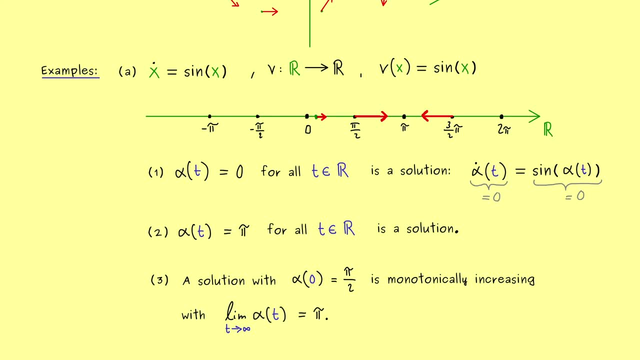 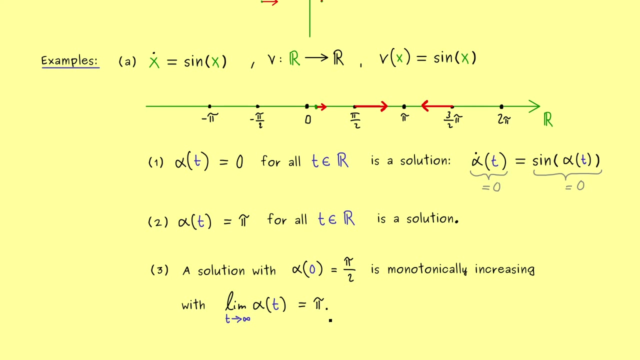 So this is very nice. So this is very nice: Knowing the explicit solution, we can already say something about its behavior. So this is the big advantage of the directional field: It helps you immediately with understanding solutions. However, maybe the whole thing is more interesting if we look at a higher dimensional example. 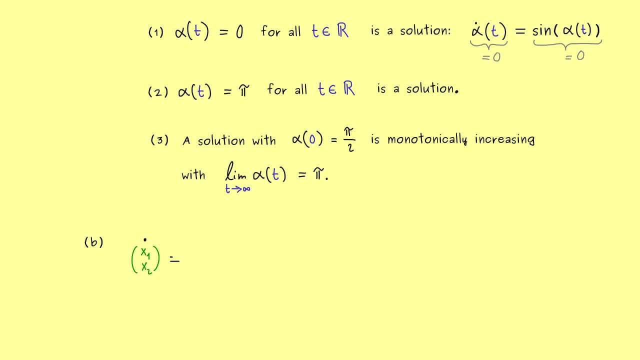 So I would say: let's take a 2 dimensional one and a similar one to the last video. So x1 dot should be minus x2.. And x2 dot should be x1.. So x1 dot should be minus x2, and x2 dot should be x8..